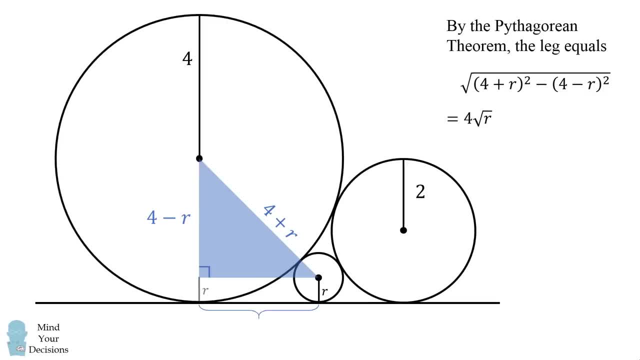 We can simplify this to be 4 times the square root of r. Now we can do a similar thing with the other circle, that is a radius of 2.. Its hypotenuse will be 2 plus r. One of its legs will be 2 minus r, and we can solve for the length of the other leg using the Pythagorean theorem. 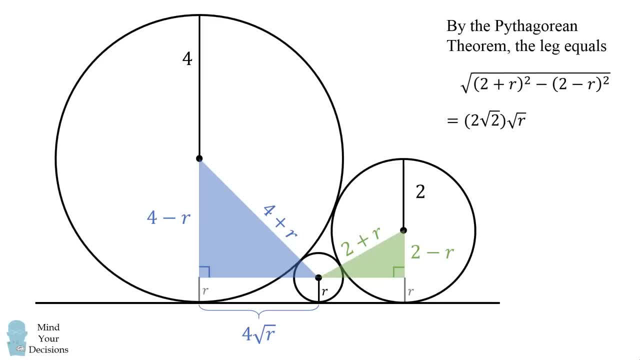 It'll be a similar calculation and we'll get. this is 2 times the square root of 2 multiplied by the square root of r. Now there's one more right triangle to consider. This will connect the centers of the two larger circles. 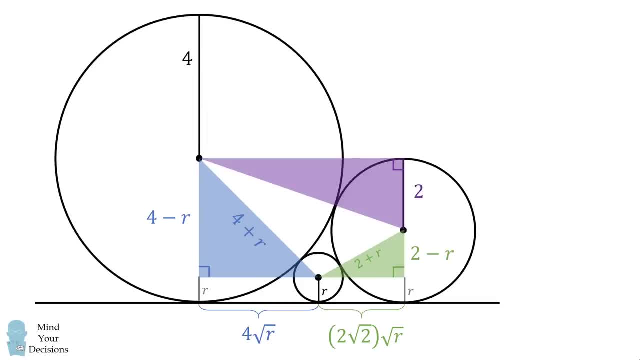 The hypotenuse will be the sum of the radii: 4 plus 2 is equal to 6.. One leg will be 4 minus 2, and that's equal to 2.. The other leg is parallel to the two lengths at the bottom. 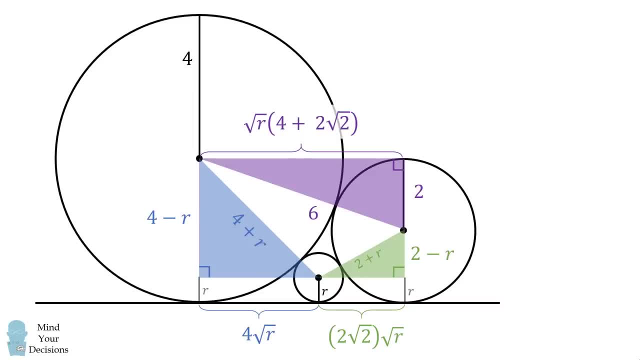 So this will be square root of r times the quantity 4 plus 2 times the square root of r. We can then use the Pythagorean theorem and we'll get 6 squared minus 2 squared is equal to the square of this other leg. 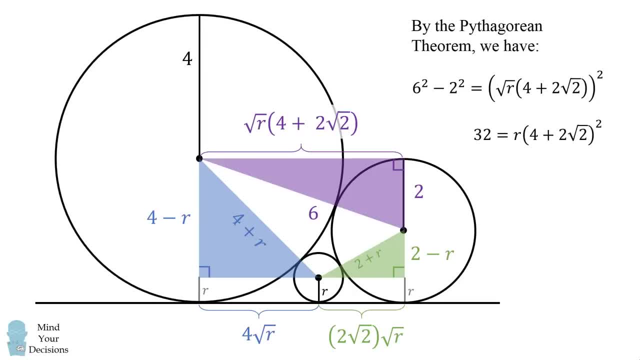 We can then do some algebra and simplify it. and now you're going to divide by 4 plus 2 times the square root of 2 squared. Now, in order to simplify that, you can multiply the numerator and the denominator by 4 minus 2 times the square root of 2 squared. 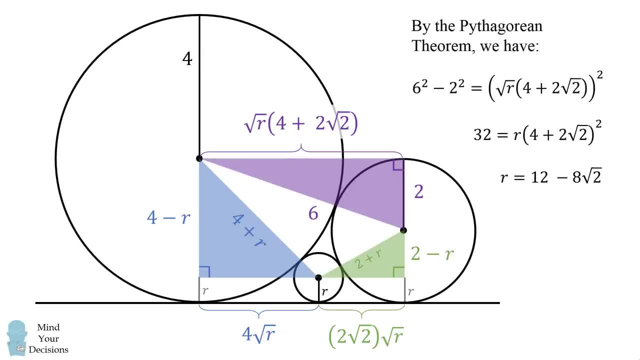 And you'll end up rationalizing this fraction and you'll get that all of this is equal to 4 minus 2 times the square root of 2. squared r is equal to 12 minus 8 times the square root of 2, and that's our answer. 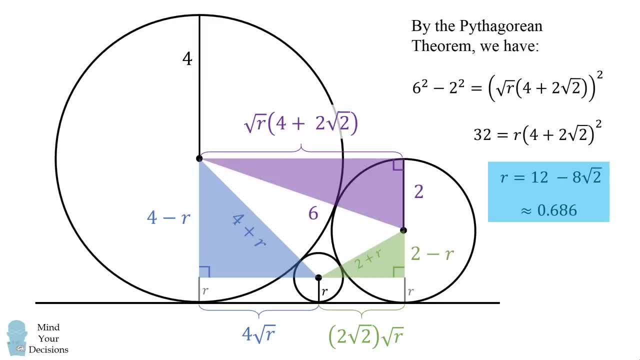 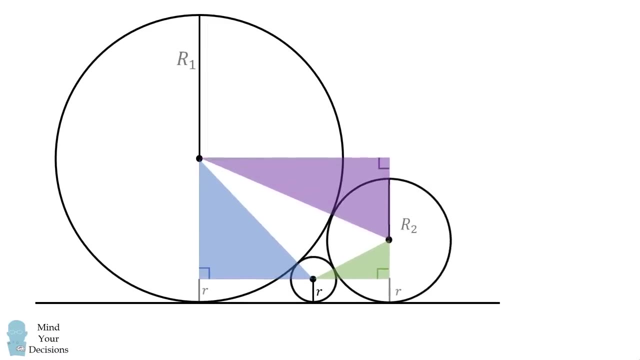 So that's our answer for these specific lengths. But can we generalize this? What would happen if our two larger circles had arbitrary values? Well, we can modify this diagram as follows. Suppose the largest circle has a radius of capital R1, and the next largest circle has a radius of capital R2.. 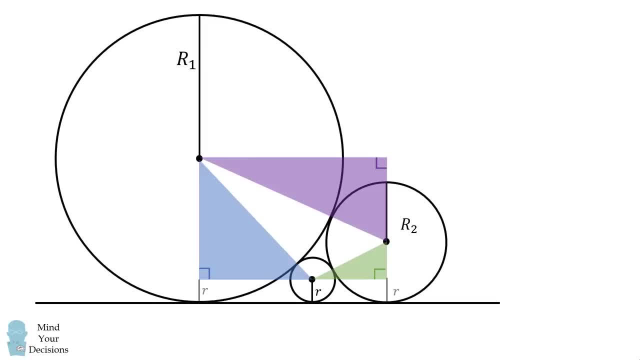 We still have the following three triangles and we can figure out the lengths of each of these sides as we just did before. The hypotenuse of each triangle will be the sum of the two radii. One leg will be the difference of the radii and we can solve for the other leg using the Pythagorean theorem. 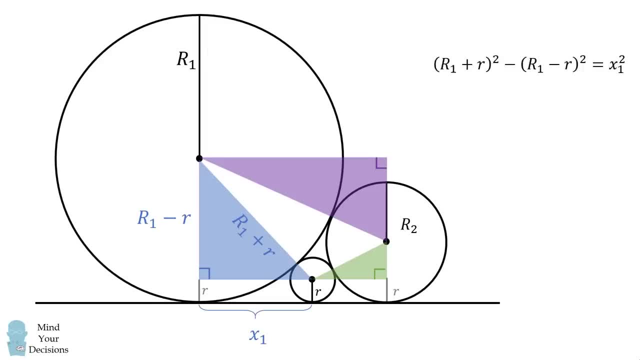 In this case we'll just label it as x1, and we could set up the following equation using the Pythagorean theorem: We'll do the same thing for the green triangle. We have x2 expressed using the Pythagorean theorem, and now in this third triangle, which is in purple, 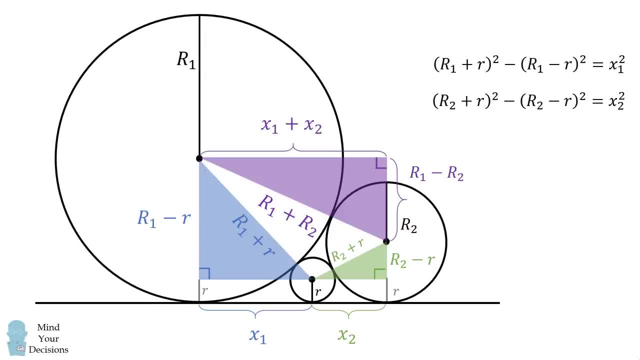 we can solve for this leg as the sum of x1 plus x2, and we can also use the Pythagorean theorem. Now, with some effort, we can solve for R, little r that is, and we'll get the following equation: 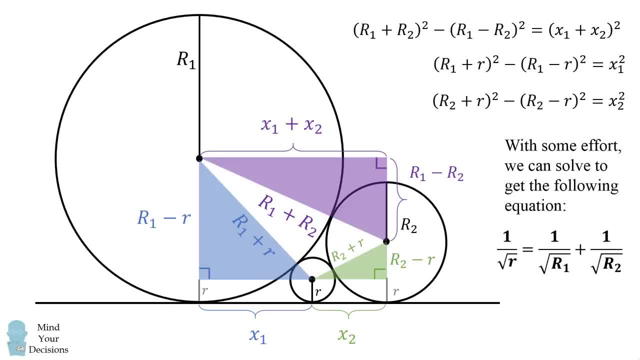 1 divided by the square root of R is equal to 1 divided by the square root of r1, plus one divided by the square root of r2.. And, like magic, we figured out an equation that we can solve for little r. 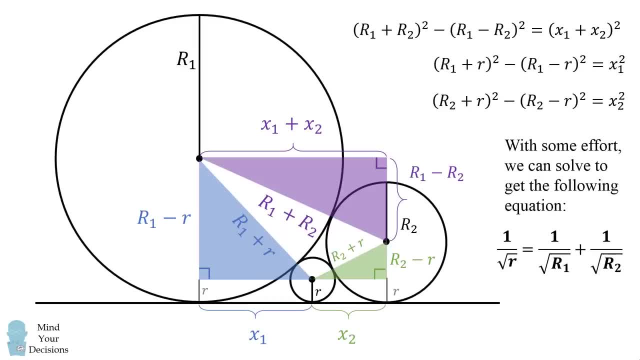 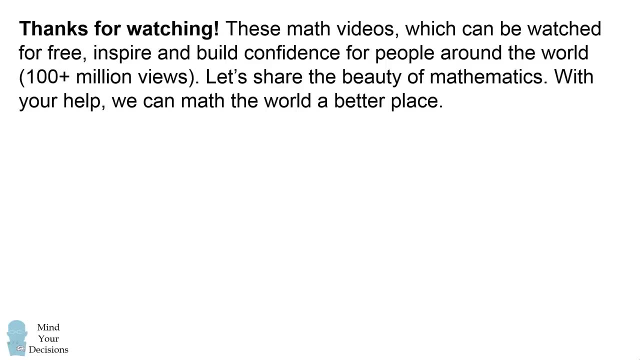 regardless of the values of big R1 and big R2.. Tremendous, Did you figure it out And did you solve for this general relationship? Thanks for watching These math videos, which can be watched for free. inspire and build confidence for people around the world. 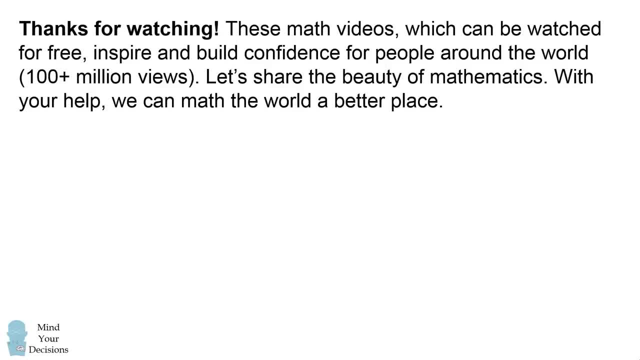 and they already have over 100 million views. Let's share the beauty of mathematics. With your help, we can math the world a better place. Please subscribe for free to get the newest videos, watch and share all of Mind Your Decisions videos. 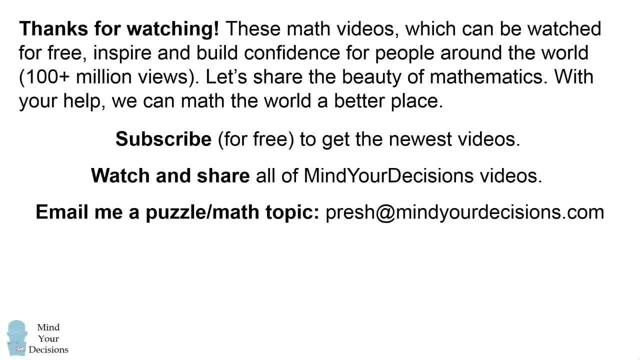 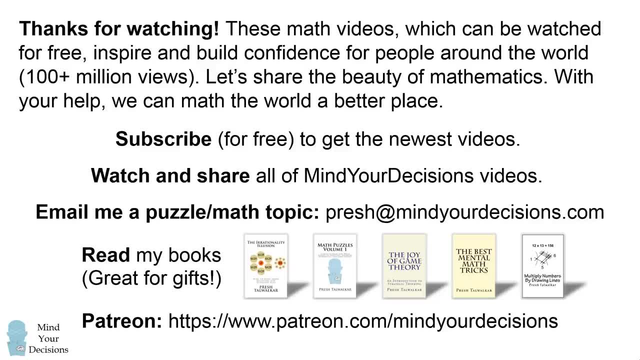 email me a puzzle or math topic presh at mindyourdecisionscom and, if you so choose, you can check out my books, which are listed in the video description, and you can support me on Patreon to earn exclusive rewards. Thanks for watching and thanks for your support.